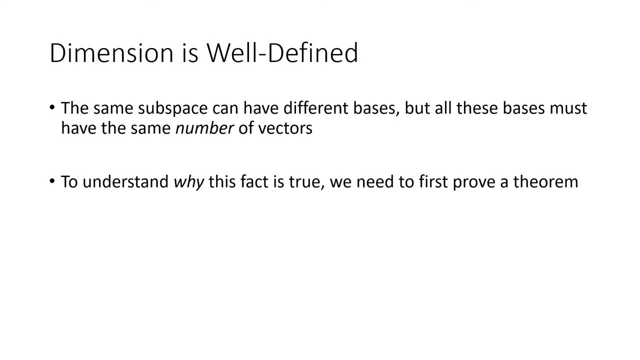 going to be talking about is the dimension of that subspace B. We wouldn't have any way of defining that, So it turns out that that can't happen Anytime. you have a subspace, any basis for that subspace, no matter what basis it is, they all have to have the same number of vectors. 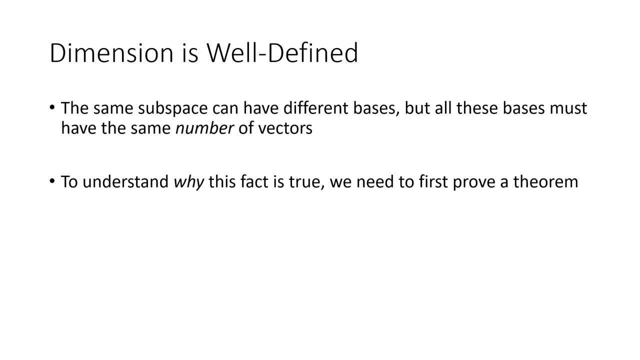 So we want to try to understand why that's true. So I'm going to go through a proof of that fact in this lecture and just try to explain how those ideas work. But before we can do that we have to prove a theorem that's going to help us do that. 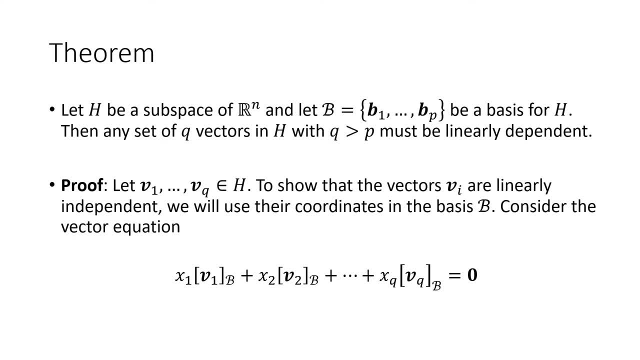 So here's the theorem. It says if you have a subspace of Rn and a basis for H, then any set of Q vectors with Q greater than P- Okay, so P here is the number of vectors in the basis. And then we're saying we have some other set of vectors, Q vectors in H, with Q greater. 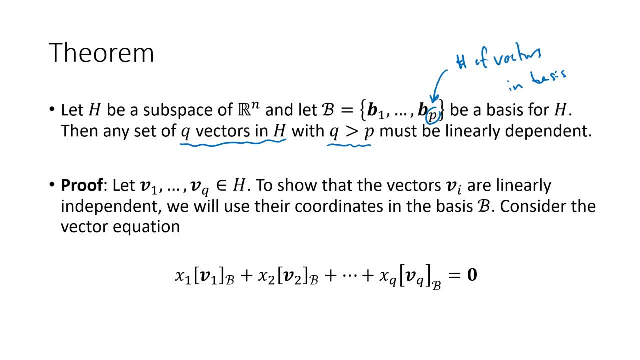 than P. So that means we have more vectors in this set that we're talking about than we do in the basis. So the theorem here says that that set of Q vectors has to be linearly dependent, In other words, there has to be a dependence relation among those vectors. Okay, so how's this proof? 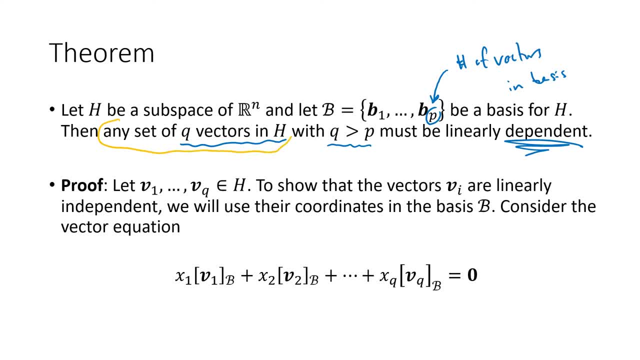 going to work. Well, this proof is about any set of Q vectors, right? The proof is saying something about that thing. So we're going to start our proof by saying: all right, let's suppose someone hands us a set of Q vectors in H, So we'll call those vectors Vs, So the V vectors, those are the. 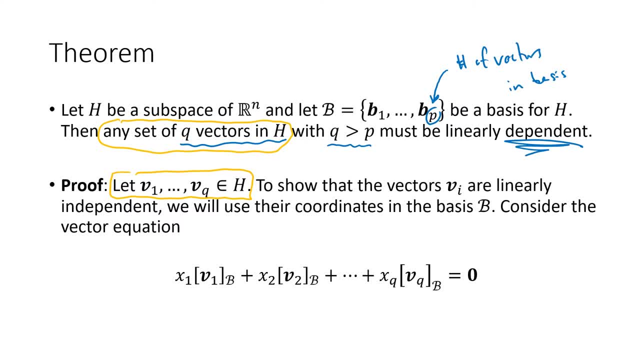 mysterious vectors, that we're trying to find out something about The B vectors. that's our basis, Which means we know a lot about it. In particular, one of the things we can do with that basis is find coordinates for any vector in H, And so that's what we're going to do. So remember this. 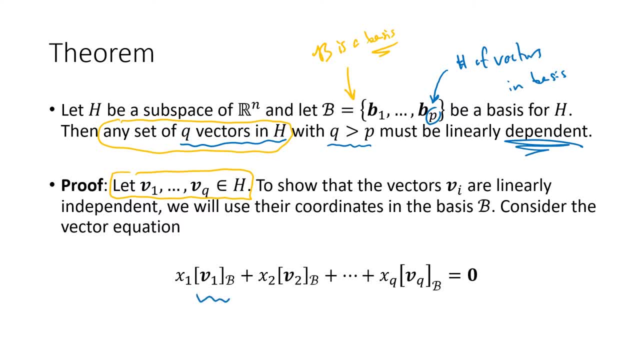 notation here. So V1 in a bracket with a subscript B, this means the coordinates of V1 relative to the basis B. So in other words we can write V1 as a linear combination of the B vectors and the coefficients, the weights that we get when we do that. we call those coordinates. 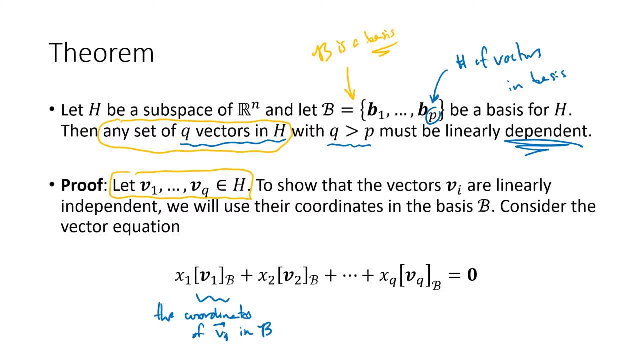 Okay, so we're going to take those coordinate vectors for each of the V vectors and write a vector equation with those vectors as the vectors in the vector equation, those coordinate vectors. All right, so that vector equation. let's think about what that is, Okay. 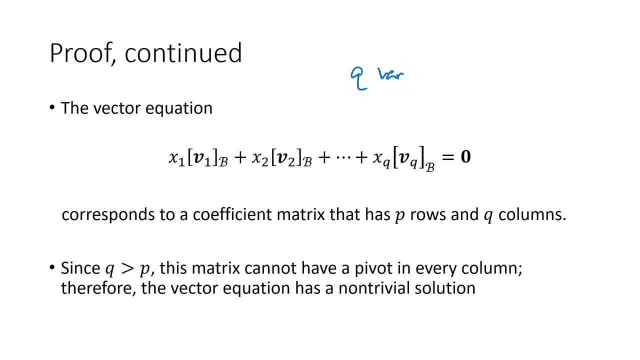 so it's got Q variables. We can see those right: X1 through XQ. But what about the vectors themselves? Well, B is a basis with P vectors in it, which means when we find the coordinates of this V vector, there's going to be one coordinate for each basis vector. 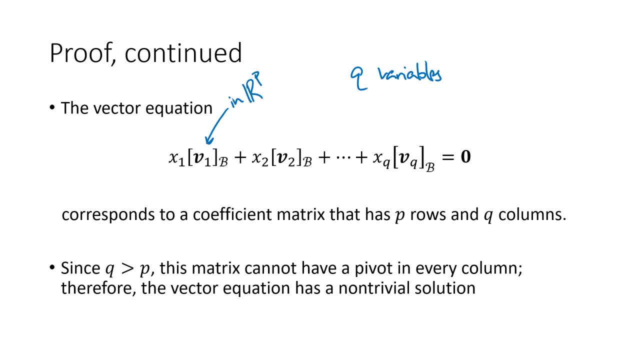 which means this vector is in RP, because we've got one coordinate in that coordinate vector for each basis vector. So the corresponding matrix for this vector equation has rows and Q columns. Let's forget the zero vector, right, So let's not worry about that. 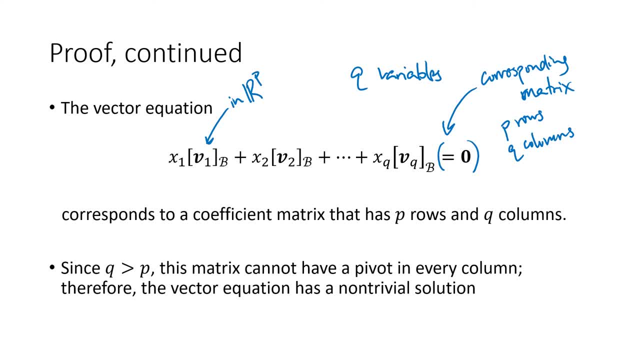 Very often when we solve homogeneous equations, we leave off the last zero column anyway. So the corresponding matrix- here we call it A- has P rows and Q columns. So in other words, the matrix equation we're talking about is: AX equals zero. This is the coefficient matrix. 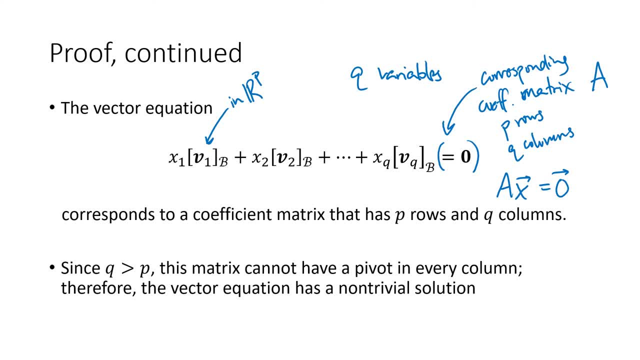 All right, so let's think about that, though We know that Q is more than P, right? This set of vectors that somebody has, we're going to call them AX and we're going to call them Q, So let's. 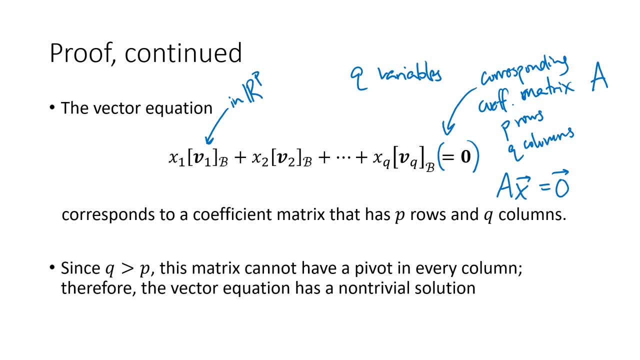 not worry about that. It means that the set of vectors that somebody else has is more than our set of vectors that somebody else has. What that means, then, is that the set of vectors that we hand to us, as that would compute the difference between the different functions, we 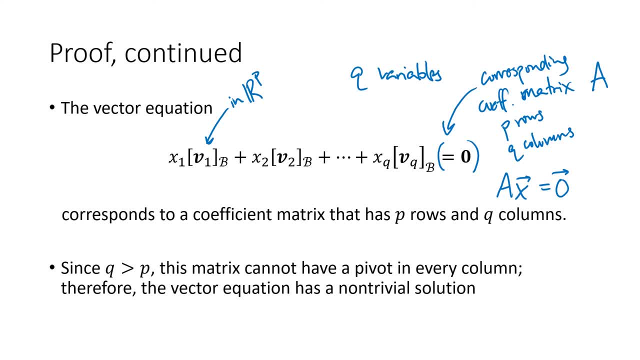 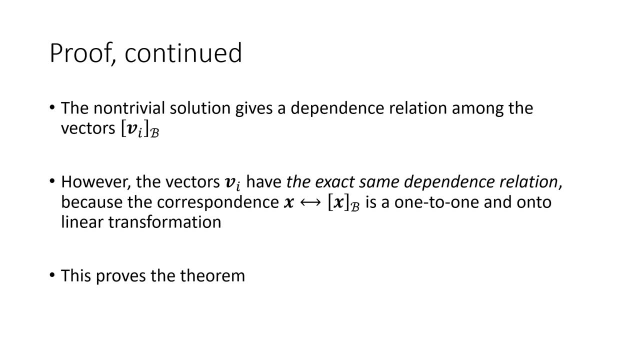 have in ourетров islast, in every column that we try to compute where we have AX value 0.. Now, on the long term, a woman, jullie hand, that we hand to us, has more vectors in it than we had in our basis, which means this matrix has more columns than it has rows. 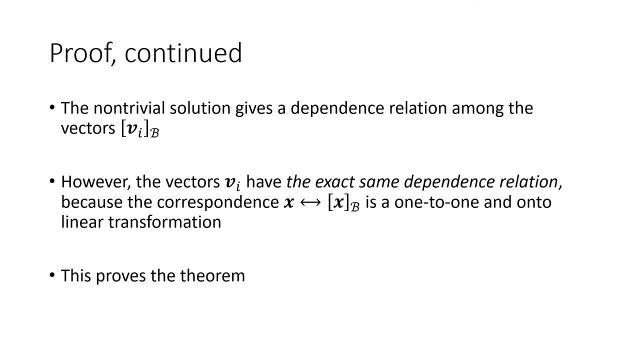 those coordinate vectors are going to have the same exact dependence relation as my original basis vectors, Because this correspondence that we talked about- if you remember, we called this an isomorphism- that correspondence is going to take those coefficients of whatever that dependence relation is and carry them back and give us a dependence relation for the v vectors, And that's. 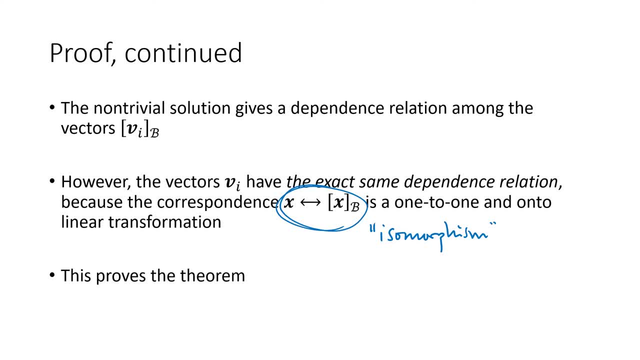 a contradiction, because the original v vectors have to be linearly independent and this would say that they were linearly dependent. So that contradiction proves the theorem A little bit abstract, but hopefully some of that made sense. Okay, so how does that help us see why? dimension? 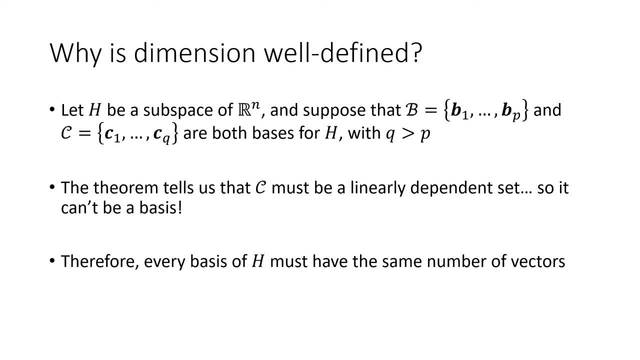 is well defined. Well, let's suppose that we had two bases for the same subspace. So in this case, let's say we had basis b, which has p vectors in it, and basis c, which has q vectors in it, And let's say that they didn't have the same number of vectors. Let's say that q was greater than p. 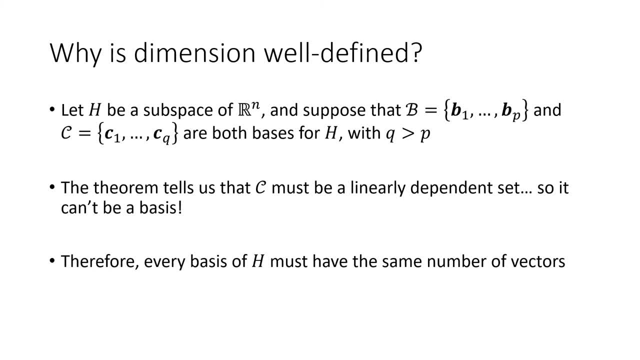 You can see how this relates to the theorem that we just talked about. Well, that theorem would tell us that c is the same number of vectors as q. So let's say that c is the same number of vectors as q. This set of q vectors would have to be linearly dependent. But wait a second. 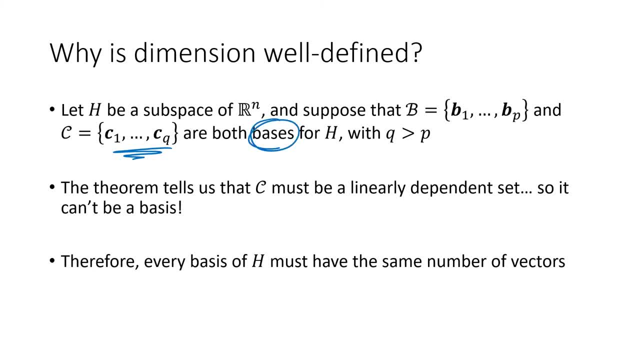 it's supposed to be a basis. Basis means that it's linearly independent. That would be a contradiction, and that contradiction means that this can't happen. You can't have two bases with different numbers of vectors in them, And so then the notion of dimension. 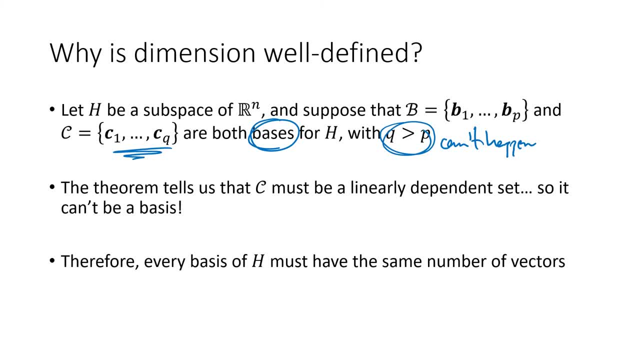 which, remember, is the number of vectors in a basis. that notion is well defined, All right, so there's more that we could say about basis. I'm not going to go through the proof of this theorem, but I'm going to go through the proof of this theorem, but I'm going to go through. 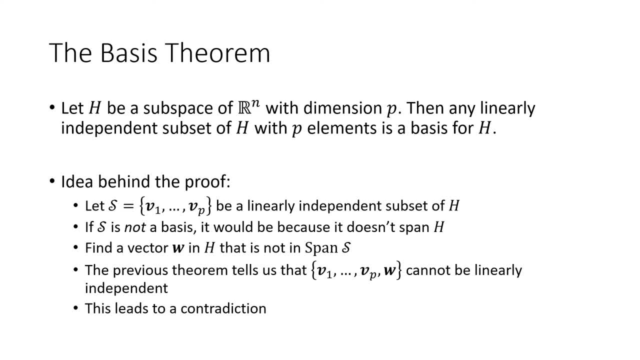 but this again gives you some more information. This says that if you have a subspace with dimension p, then any linearly independent subset of h with p elements- so it's a linearly independent set- it's got the right number of elements. that turns out that that's enough to. 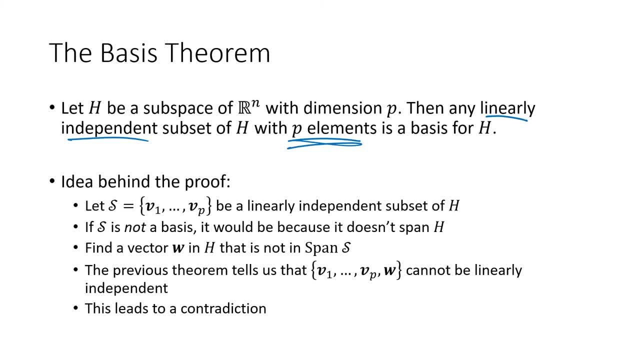 say that it's a basis. In other words, we wouldn't have to prove that this set spans this subspace. And I've got some bullet points here to sort of walk you through the proof. but again, hopefully that makes some some sense to you. Okay, a couple other definitions. So if we have a matrix, 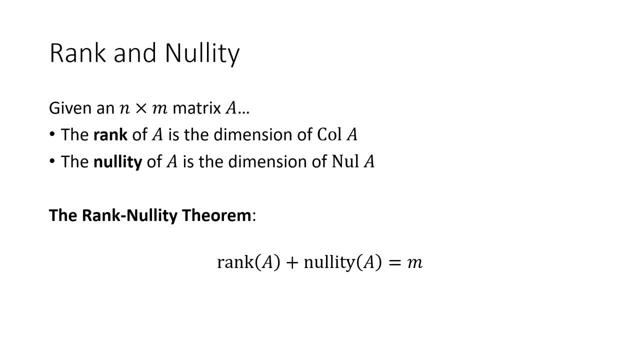 n by m matrix, n rows, m columns. the rank of a is the dimension of the column space of a, So that's just a special name for the dimension of that special subspace. The nullity of a is the dimension of the null space of a. So, again, just a special name for the dimension of that special subspace. 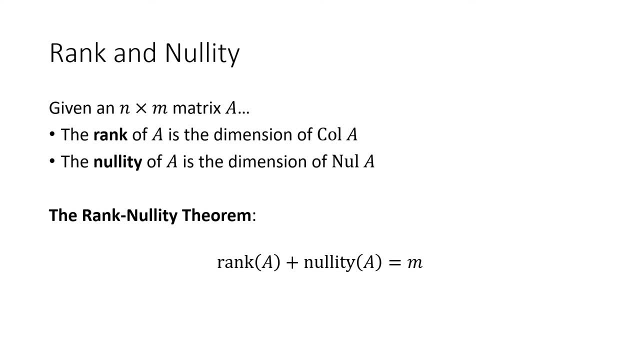 And it turns out that we have this nice relationship called the rank nullity theorem, which says that if you take the rank of a and add it to the nullity of a, then what we get is m, which is the number of columns of a. 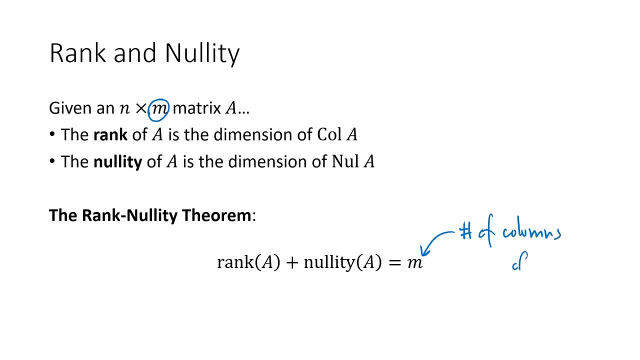 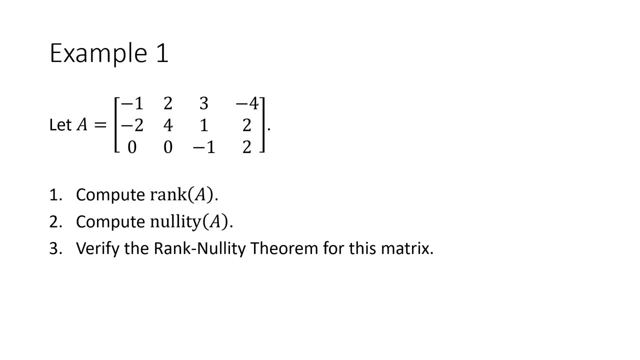 Now I could go through a proof of this for you, but it's actually pretty easy. and to show you why, let's go through an example. All right, so we have a matrix here and what I want you to do is compute the rank, compute the nullity and then verify the rank nullity theorem. So remember this matrix A. 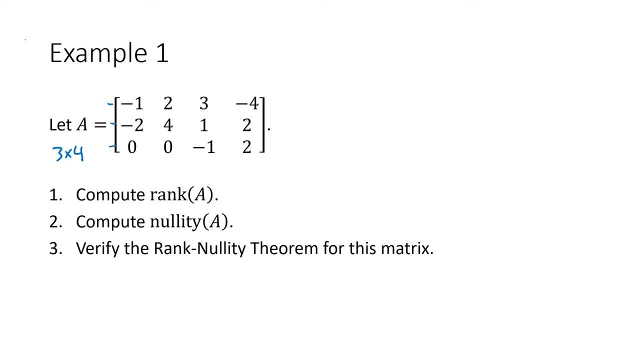 is three by four, We can see that it's got three rows and four columns. So what I'm going to do is I'm going to row reduce this matrix. Remember that to find an actual basis for the rank nullity theorem, both of those require us to row reduce this matrix. So we're going to row reduce A. 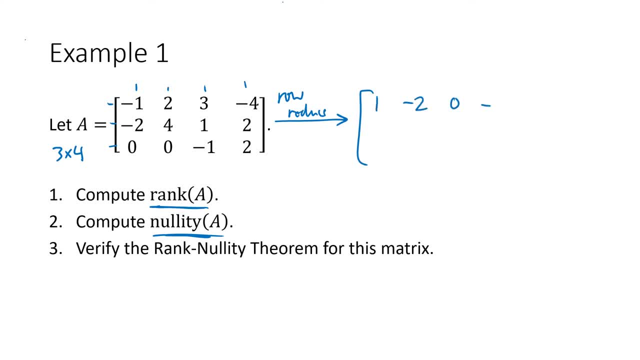 and in this case it turns out to be one negative, two zero negative, two zero zero, one negative, two zero, zero, zero, zero. Okay so let's think about rank. So remember, the rank is the dimension. 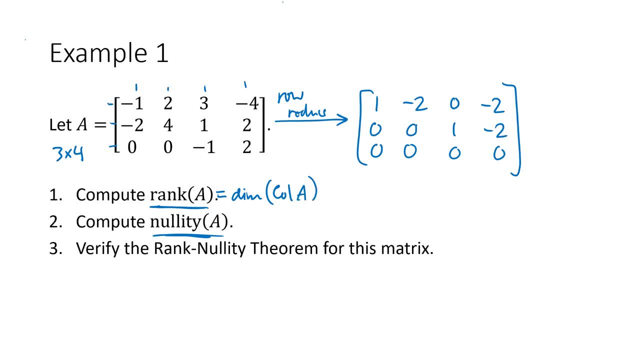 of the column space of A. But if we actually wanted to find a basis for the column space of A, what would we do? Well, we would try to find the pivot columns of A, and we can see that when we row, reduce our matrix, the first and third columns have pivots, and that means that 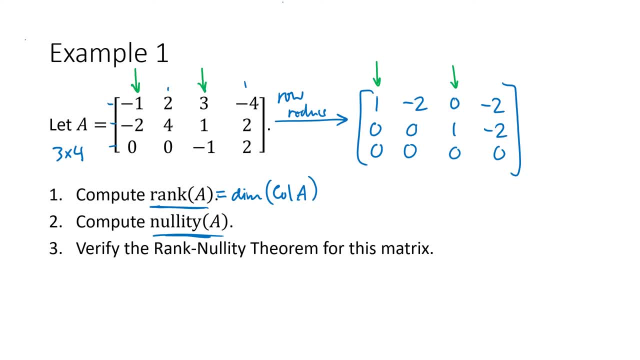 the first and third columns of A are the pivot columns of A and that means that this dimension is the number two, because that basis we can actually see the basis. it's right here. this vector and this vector, these vectors have circled in green, those vectors are the basis. 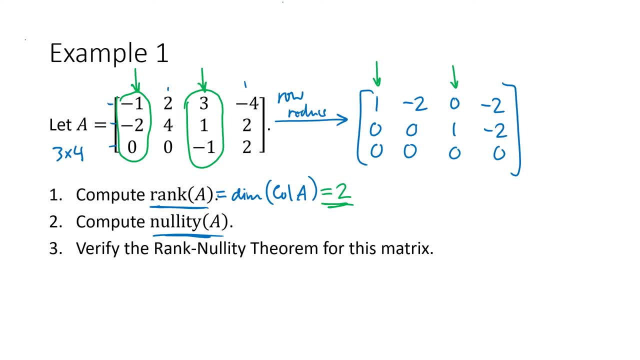 for the column space of A, and it's got two vectors in it. so that means dimension is two. What about the nullity? Well, to find the nullity, it's not quite as obvious, but what we need to do is solve. 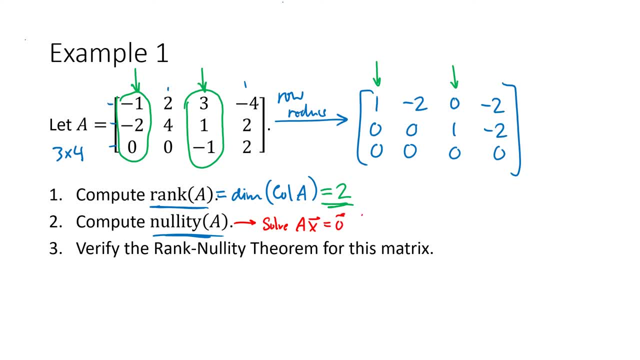 Ax equals zero and look for the number of free variables. Remember that when we find our solution to Ax equals zero and write it in parametric solution form, the number of free variables is going to tell us the number of vectors that we get. 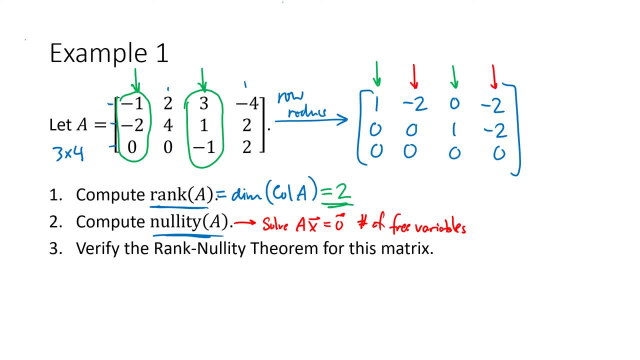 Well, the number of free variables corresponds to the number of non-pivot columns in our row. reduce matrix. This means that x2, which corresponds to that column, and x4, which corresponds to that column, those are going to be my free variables when I go to solve. Ax equals zero.